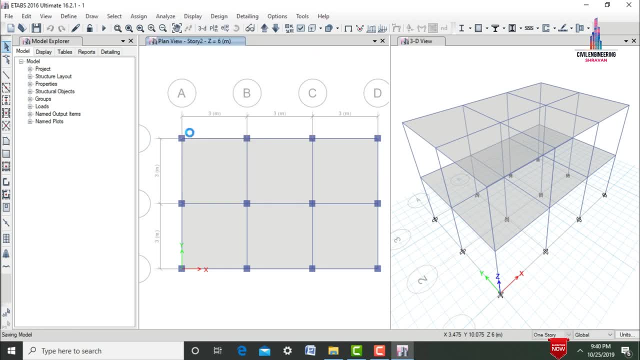 to analyze option here. So here we need to select run Open analysis option. So run the analysis for this respective G plus one building. So this is my deformed shape for the respective G plus 1 building due to presence of the dead load case, so click on start animation. So this is the animation for this respecto building. 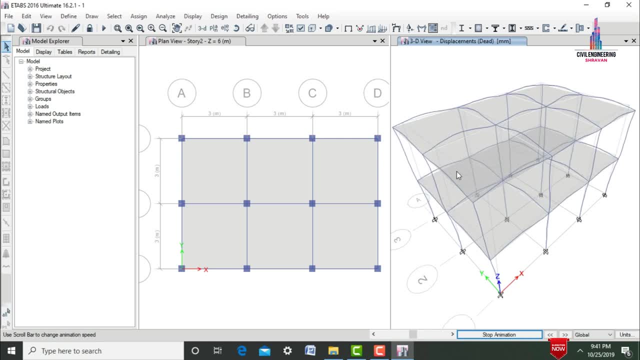 due to presence of the dead load case. So I will change the dead load case to live load case. So for that go to display option here. So I selected that, just select all Ich. so this enough. so final check models here Here you can see my test client files So you can. 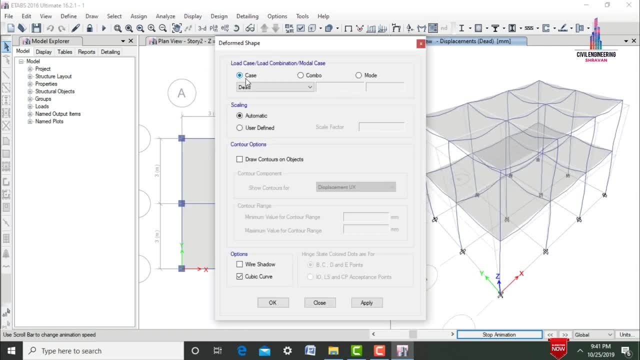 see a little bit. I just saved all the calculations and our test warrior boards. So this is now ready in the test builder bereit most. So get your test which you want to test. your test Iman can out d-palm shape. so here we need to select the case. nothing but the selection of load cases. 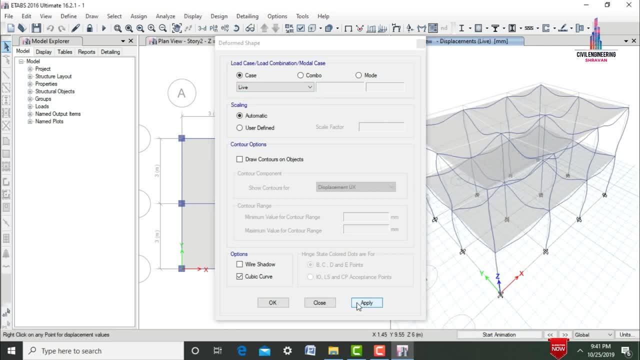 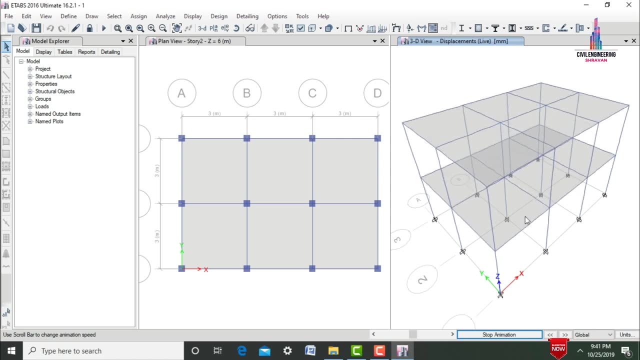 just i'm selecting it as live load case. click on apply. click on ok again. select your stat animation. so this is the deflection diagram for this respective structure, due to presence of both load cases: dead load as well as live load. so, after checking the deflection diagrams, we 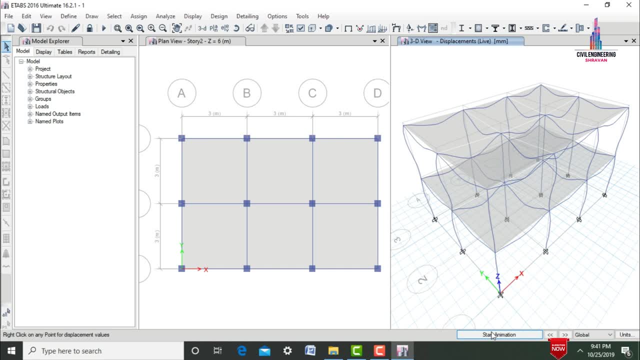 need to check the shear force diagram, bending moment diagram, as well as the building torsion values for this respective building. so for that initially go to display option here. so here we need to select the four stress diagrams. so in the four stress diagrams we need to select frame. 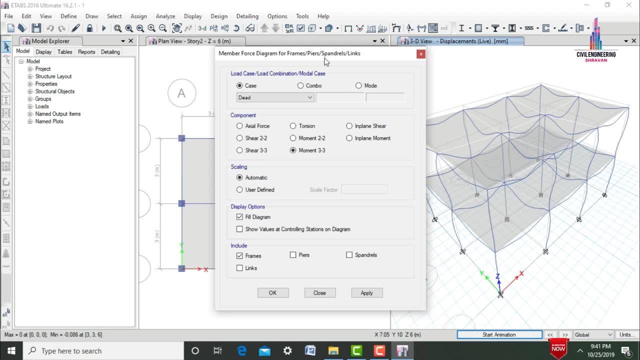 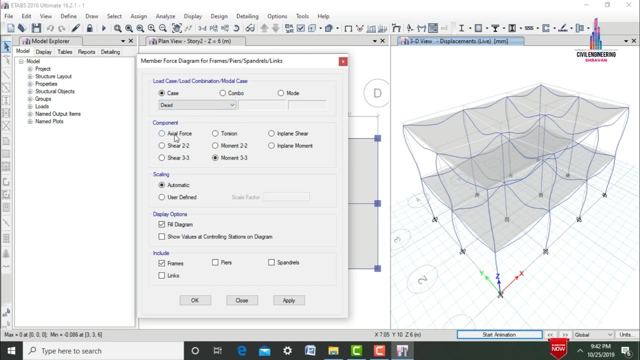 pierce spandrel forces here. select this option. so here we need to select any one of the load cases. just i'm selecting load case as dead load case. so initially we need to select axial force component. click on apply. so this is the axial force diagram for this respective building due. 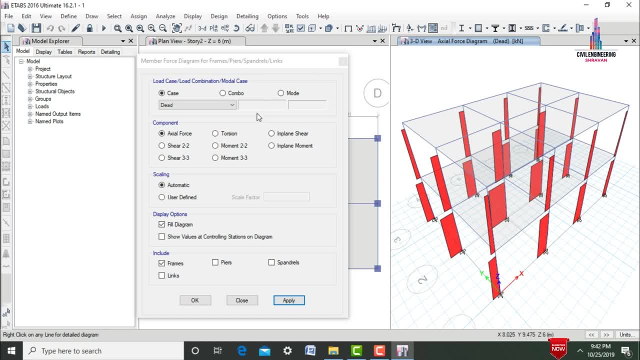 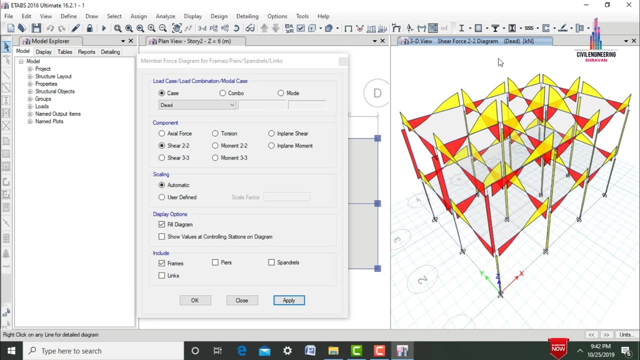 to presence of this, this respected dead load case. so after that, just i'm selecting the shear, click on apply button. so this is the shear force diagram for this respected structure, due to presence of this respected dead load case. so after that we need to select the bending moment diagram. so select bending. 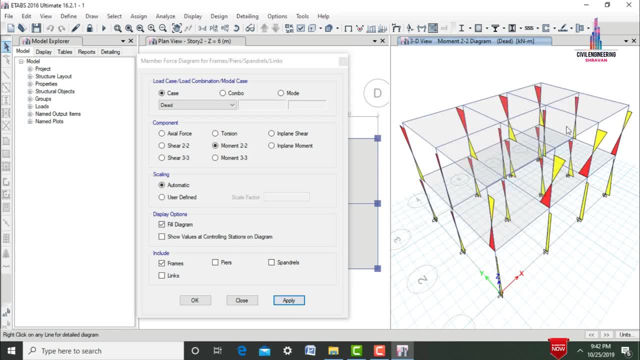 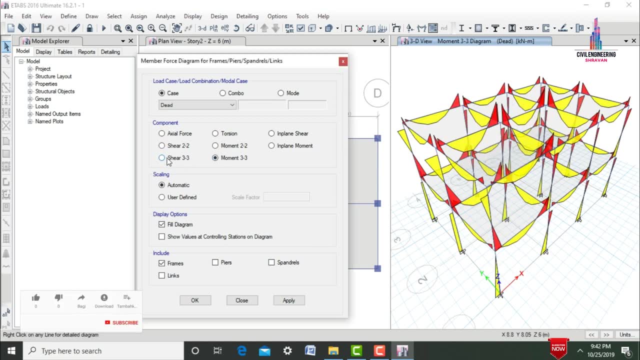 moment diagram. click on apply. so this is the bending moment diagram in x direction. select bending moment diagram three three. click on apply. so this is the bending moment diagram in y direction. so after that we need to select shear three three. click on apply button. so this is the shear force diagram in y direction case. so i am selecting torsion option. 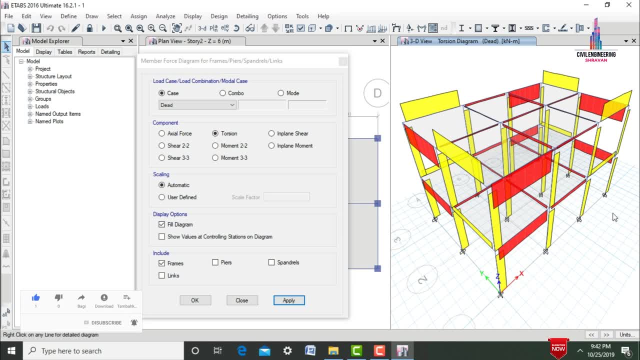 here. finally, click on apply. so this is the building torsion for this respected structure due to presence of the dead load case. just, i'm changing the dead load case to live load case. here again we have to apply apply button. so this is the building torsion diagram due to presence of the live load. 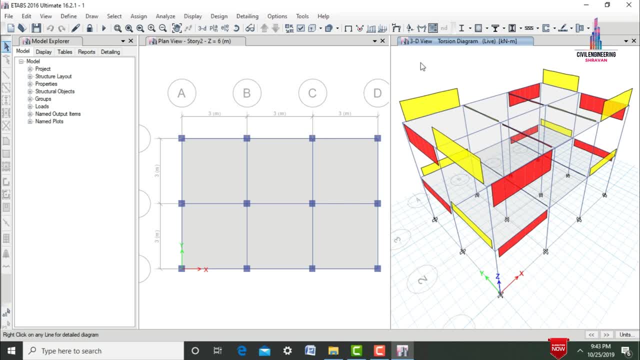 case. so after that, click on ok button. so again select this respective 3d model. click on display option: select your undeformed shape. so, after checking the deflection value, shear value, as well as bending moment values and torsion values, we need to design this respected building. so for that, go to design option. 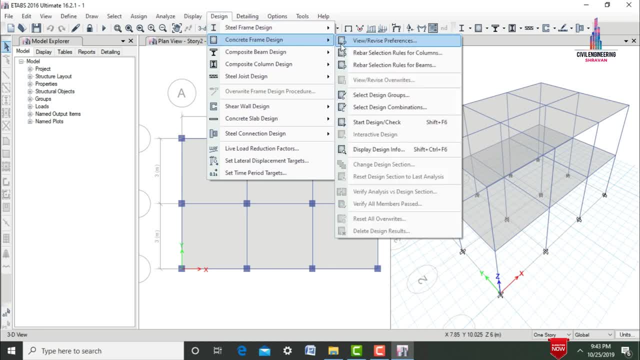 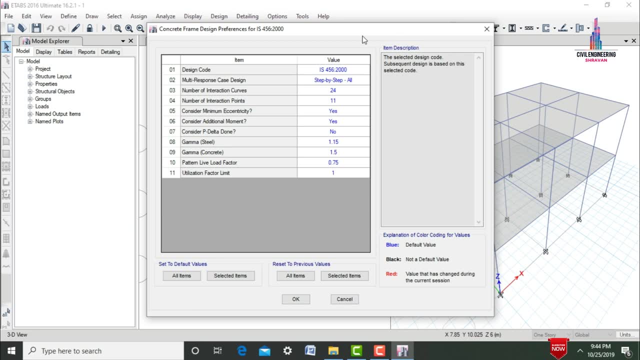 here select your concrete frame design. so here we need to select the view revised preferences initially, this time selecting view revised preferences. so it will be consisting of design code, of is456 code and a number of intersection curves are 24 and number of intersection points are 11. so it is consisting of gamma of steel is 1.15 and gamma of concrete will be a 1.5. 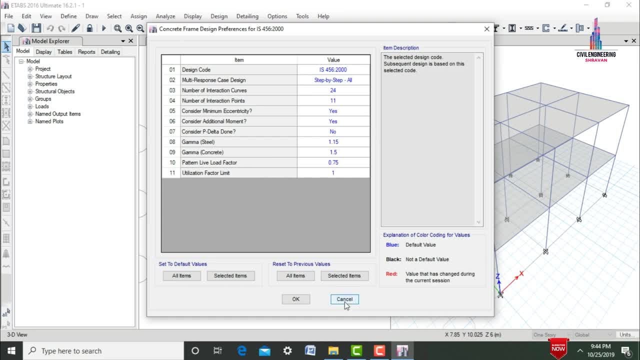 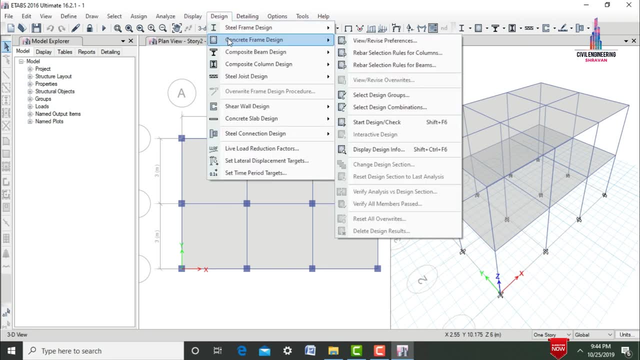 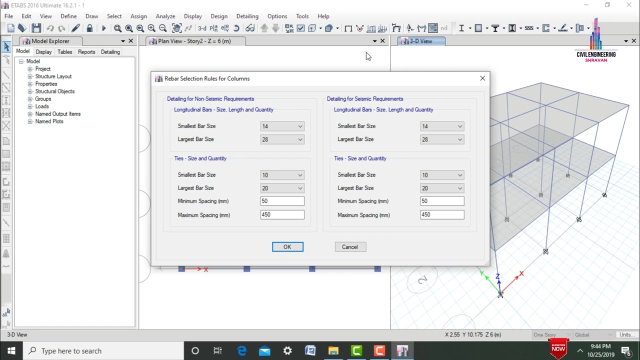 which is nothing but your safety factor. so select your ok button here. so after that go to design option. here again, select your concrete frames design. so we need to select the rebar section. rules for the column. initially, just i am selecting rebar section for the column, so it will. 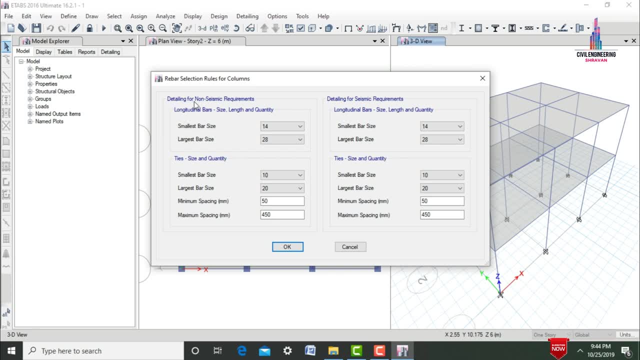 be consisting of two parts here. the left hand part will be consisting of details of non-seismic records, like the column design. then it will be consisting of details of non-seismic records, and right hand side section will be consisting of details of seismic requirements. so for this, 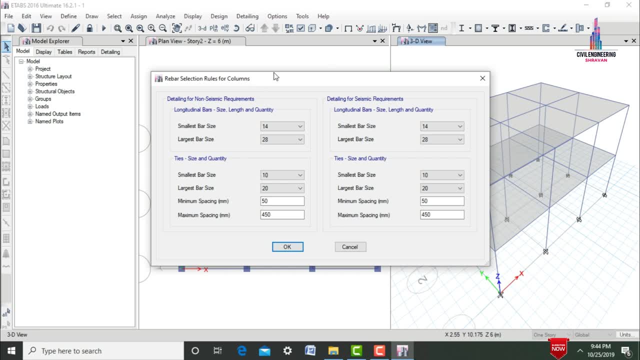 respected building. just i am assuming a non-seismic case, so for that we need to select the left hand portion for this respected selection option. so in this part of non-seismic case it will be consisting of small bar size and larger bar size and it ties dimensions. just i am selecting small bar size will. 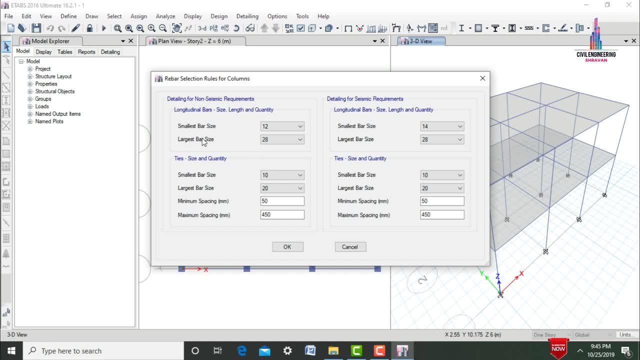 be consisting of 12 mm. after that we need to select larger bar size. just i am selecting it as 16 mm, so after that we need to select the ties. so just i am selecting a smaller bar size will be consisting of 8 mm bar. again i am selecting larger bar size will be consisting of 12 mm for this. 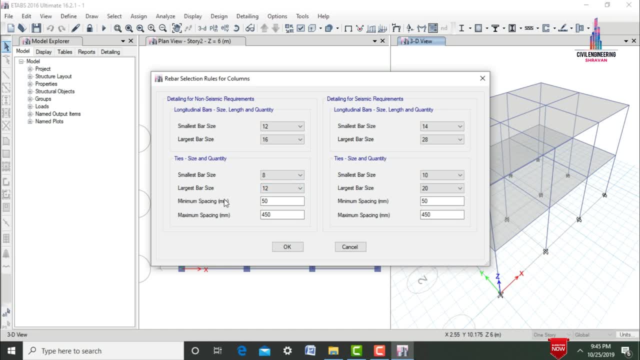 respected column section. so here i am assuming a minimum spacing will be 50. after that we need to assume maximum spacing. just i am assuming maximum spacing is 300. click on ok, okay, okay. after defining the rebar section rules for the column, we need to define the rebar section rules. 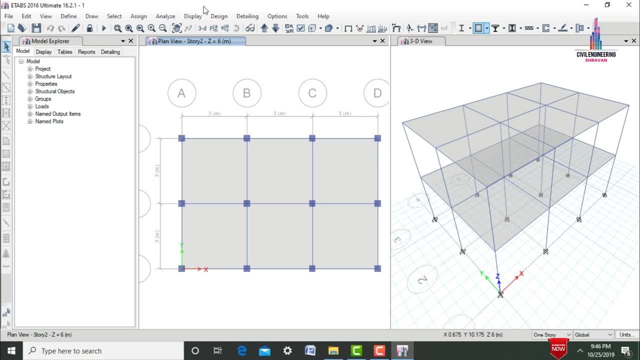 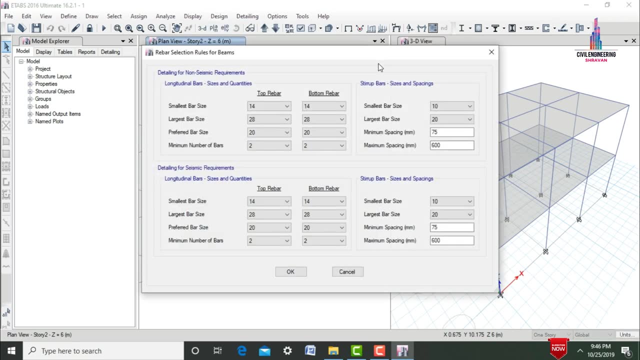 for the beams also. so for that again go to click on design option. so here we need to select the concrete frame design. here we need to select rebar section rules for the beam section. so it will be consisting of two parts, which is of non-seismic case and a seismic case here. so here i am selecting. 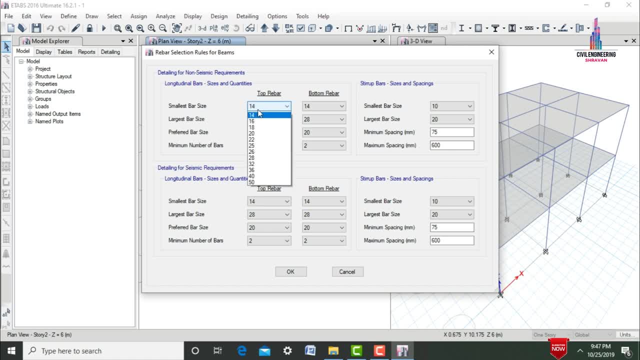 non-seismic case. just i am selecting: small bar size will be consisting of 12 mm for the beam section, for top reinforcement as well as bottom reinforcement. so again we have to assume the larger bar size. just i am assuming larger bar size will be consisting of 20 mm. here again i am selecting. 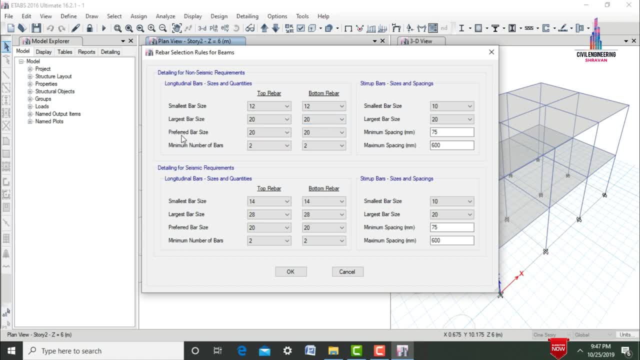 bottom larger bar size of 20 mm. so after that we need to select preferred bar size. just, i am assuming preferred bar size is 16 mm for this top reinforcement. again, i am selecting 16 mm for bottom reinforcement, so after that we need to assume the minimum number of bars for top reinforcement as 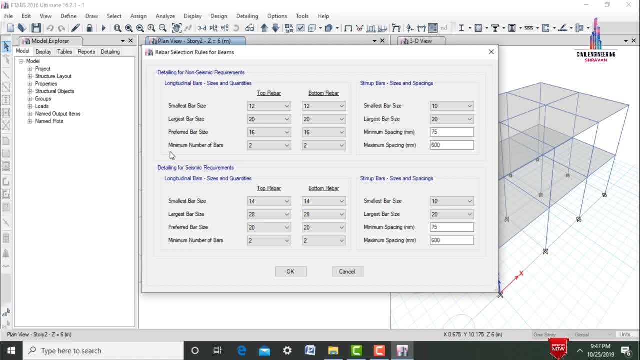 well as bottom reinforcement, as per my assumption. just i am taking it as 2 and 2, so after that we need to select the stirrups data here. so here i am selecting small bar size of 8 mm. again i am selecting maximum bar size of 10 mm, so after that we need to assume the minimum spacing of 75. so 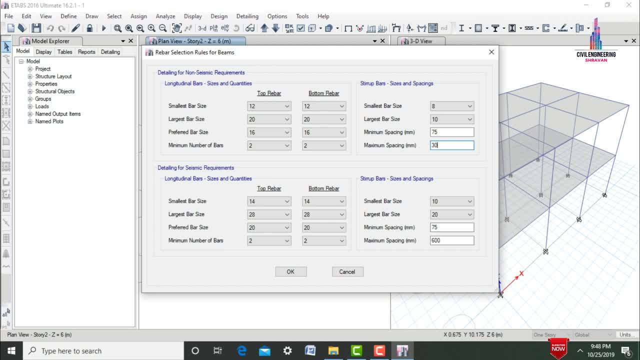 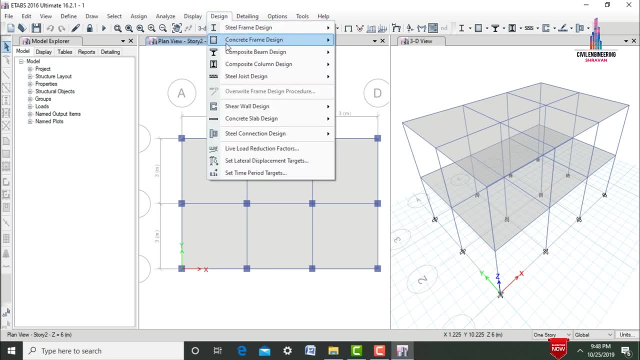 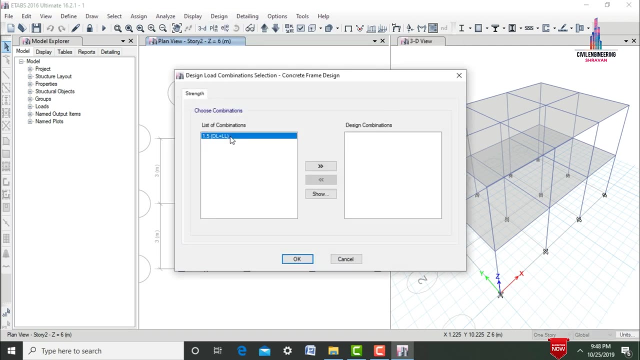 just, i am taking the maximum spacing option as 300. click on ok option. so after that we need to select the load combinations for designing. so go to design option here, concrete frame design. again select your select design combination. so here we need to select this respective option. 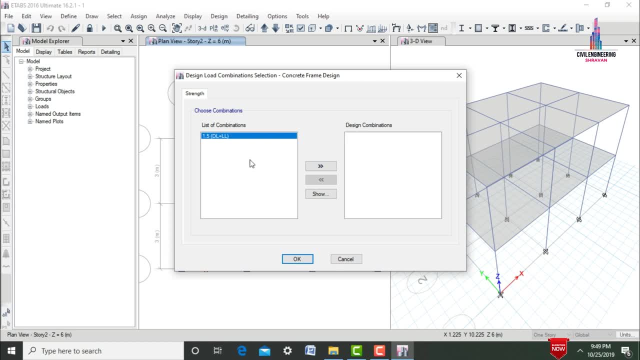 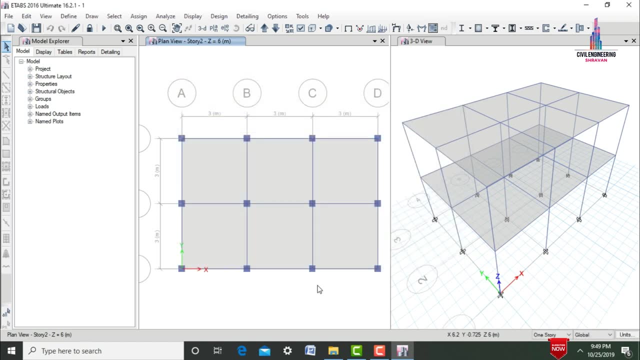 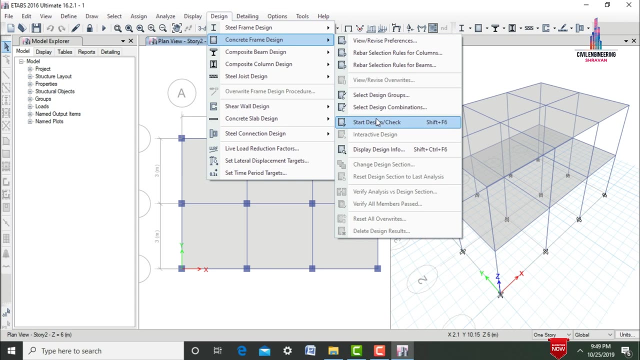 which is consisting of 1.5 times of dead load plus slide load option. so include your load combination. click on ok option. so after that we need to design this respective model. so go to go to design option. here select your concrete frame. so here we need to select the start design. 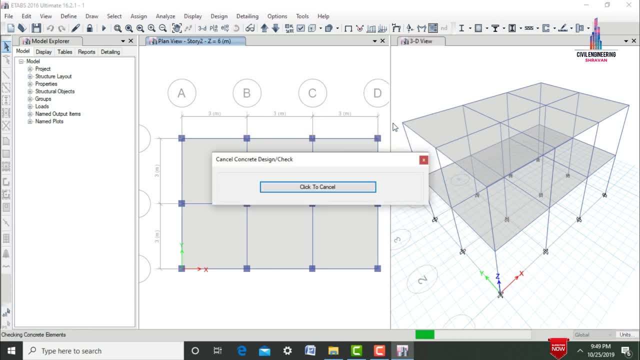 check. select this respective option. so it will start designing the respective model like this. so this is my reinforcement: percentage values for the respective beam section at different levels. so i will show you this respective diagram in 3d view. select your 3d option. so this is my. 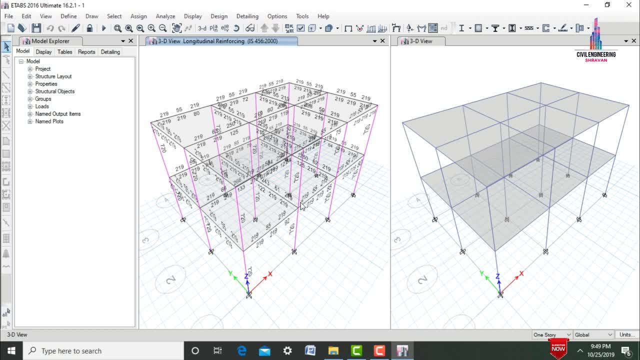 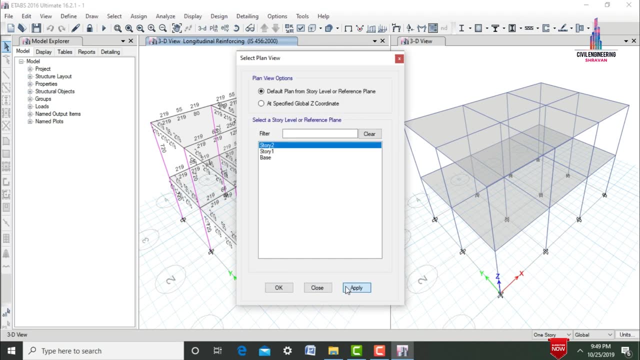 reinforcement values, percentage for the respective beam section as well as column section, at different levels. so after that i am selecting in plan view, which is of second story. click on apply here. click on ok. so after that we need to check the values of the reinforcement details for the beam as well as. 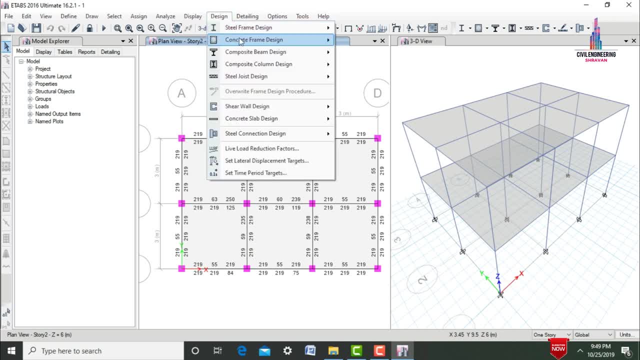 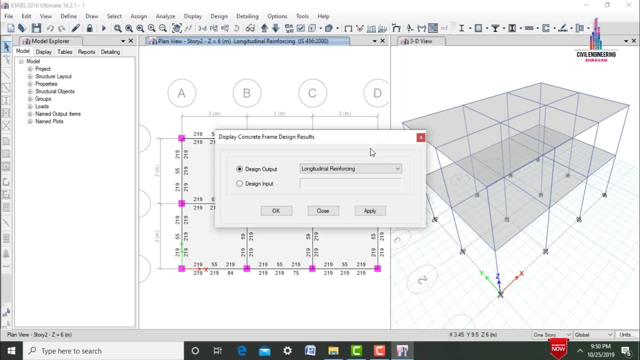 that initially go to design option. here again we have to select the concrete frame design. so here we need to select the display design information. so here we need to select the design output value. so just, I am selecting shear reinforcing. so click on apply, click on ok, so it will show you the values of the. 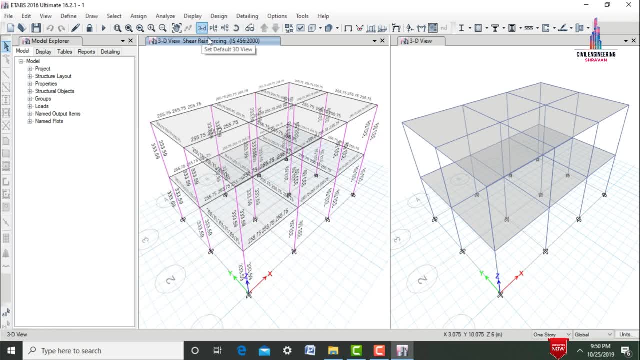 shear reinforcing for this respective model. so click on 3d view. so this is the shear reinforcing values for the each and individual beam section, as well as each and column section for this respected G plus 1 building. so after that we need to check the values of the beam reinforcement values- column. 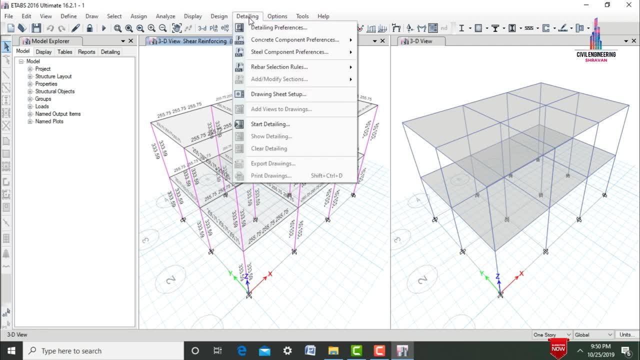 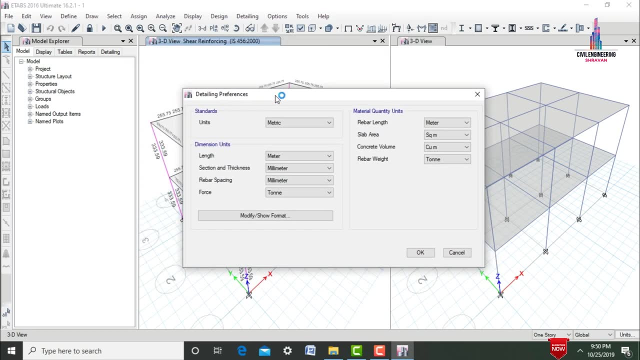 reinforcement values. so for that, initially go to detailing option. so here we need to select the detailing preferences initially. so here we need to select some options which is related to designing data. so here I am selecting: units will be in metric system and length will be in meter, and the section 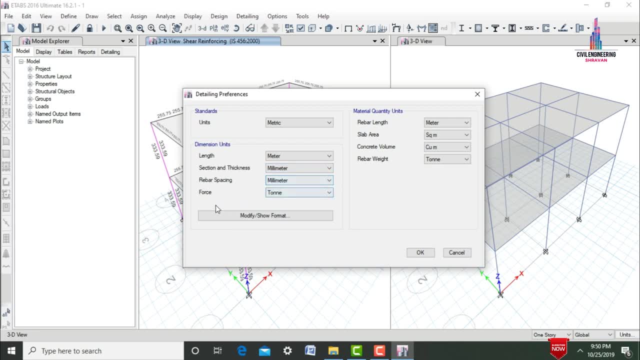 and thickness will be in mm and rebar spacing is also mm. so here I am selecting. 4 will be in kN, so after that we need to select the material quantity units. next time, selecting rebar length in meter and slab area will be in square. 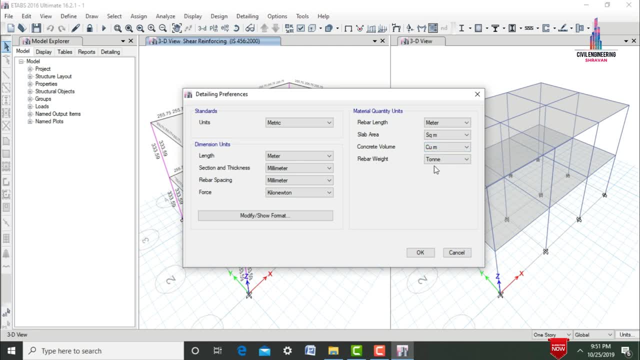 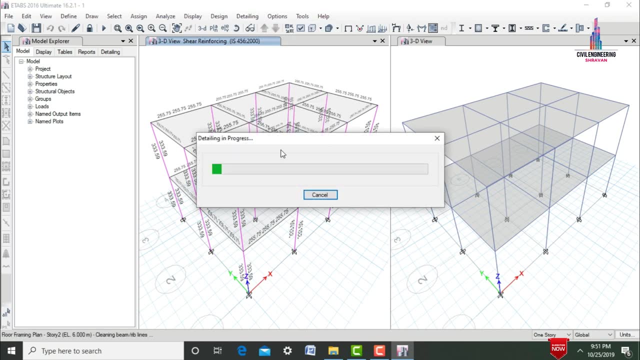 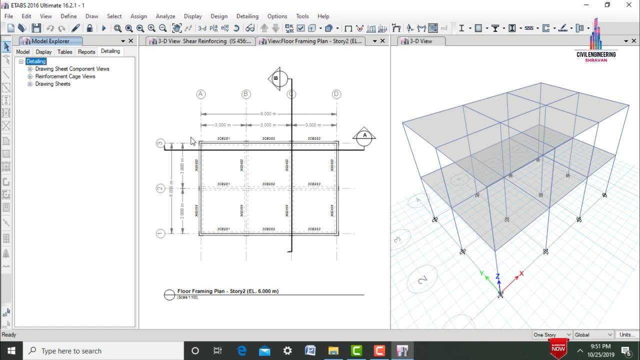 meter, concrete volume will be in cubic meter and rebar weight will be in ton. click on ok. so after that, click on detailing. so here we need to click on start detailing option so it will detail the respective options like this. so this is the plan view for this respected. our second story, for the respected elevation: 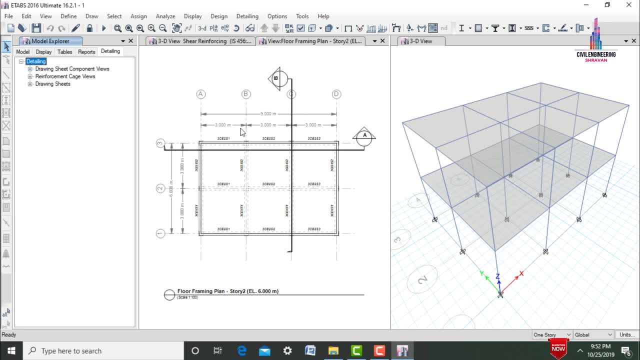 of 6 meter height. so this is a center-to-center distance for the beams and column section. so after that we need to check the values of the beam reinforcement, column reinforcement. so here we need to select this respective standard details. so in the standard details we need to select typical concrete beam elevation 2s. just double click on it so it will. 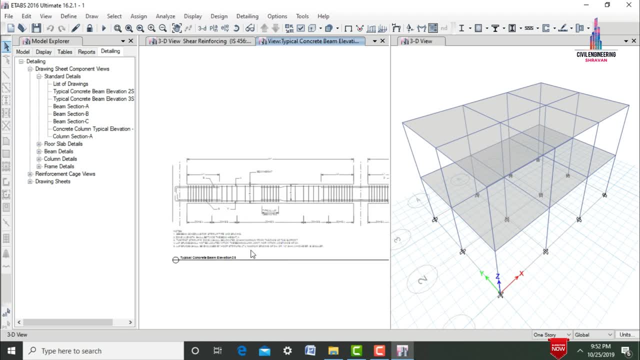 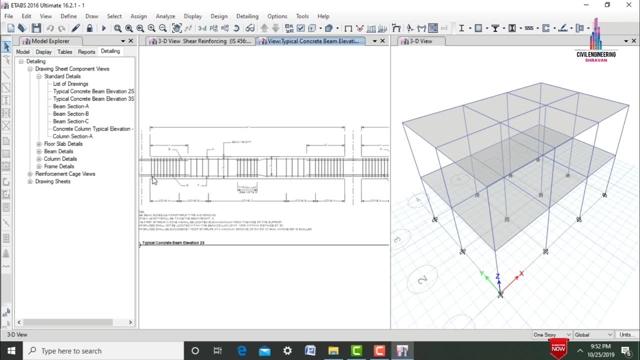 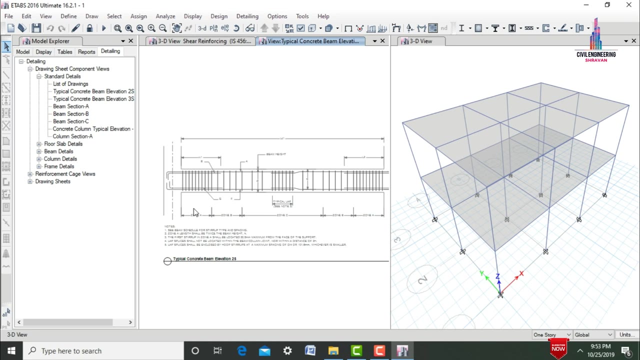 show you the typical diagram of the respected beam section here like this. so this is the typical beam section diagram for this respective model, which is consisting of some zones here, which is of zone A, Zone B, Zone C, as well as Zone B and Zone A here. so here, zone A in left hand side. 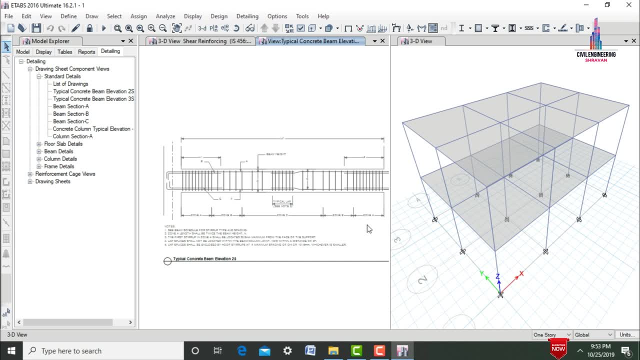 section, as well as zone A in right hand side section, is the corner values of the respected reinforcement values for the beam section. so zone B. Zone B is the intermediate value, so zone C is the center value of the reinforcement for this respected beam. so this is the values of the 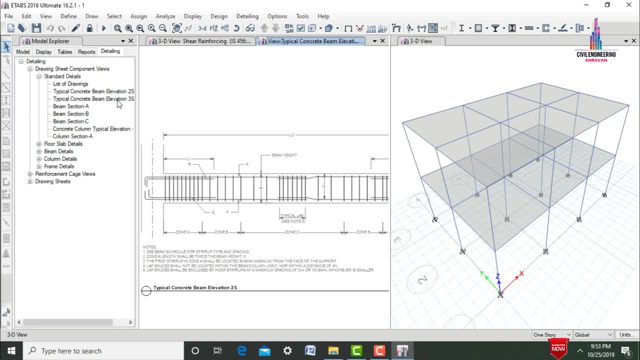 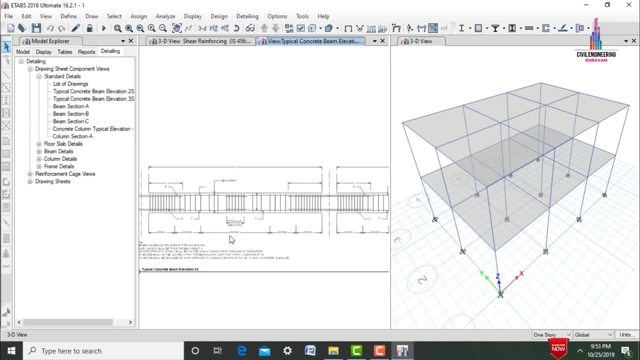 beam design results for typical 2s section. just, I am selecting concrete beam of elevation 3s section. So this is the three column sections, which is also consisting of zones here: zone A, zone A, zone B, zone B, zone C. So select your respective beam section. 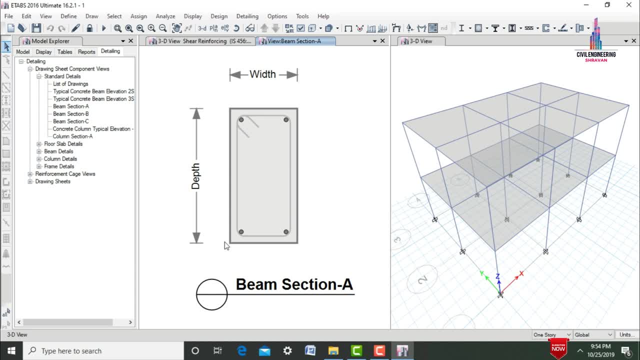 So just double click on it. So this is the beam section AA for this respected zone A section. So select your respective beam section B. So this is the diagram of reinforcement for the beam at B section. select the beam section of CC. So this is the diagram for the respected beam section C. 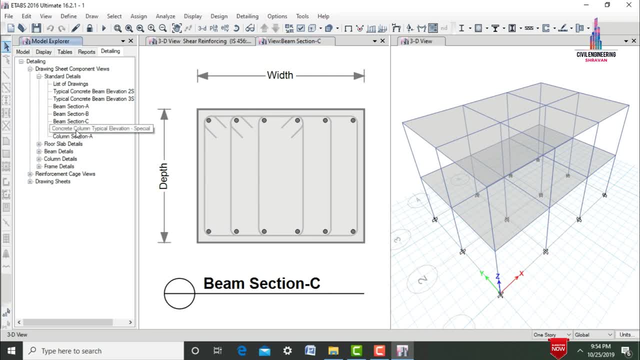 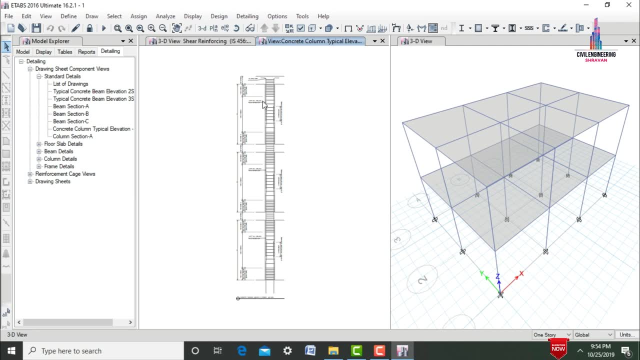 So after that, select your column typical elevation. just double click on it. So this is the typical column elevation for this respective G, plus one storey building for this respected column. So this is the column typical elevation for this respective case. So after that we need to select the column. section A dimensions. 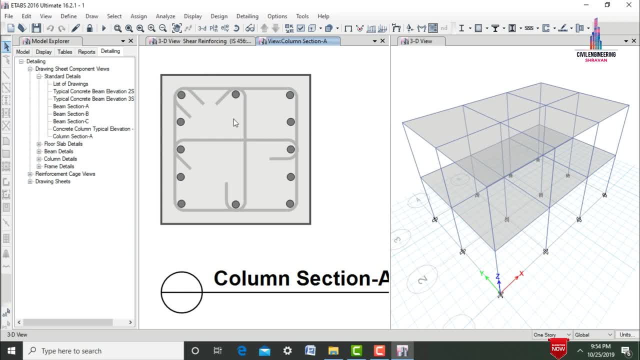 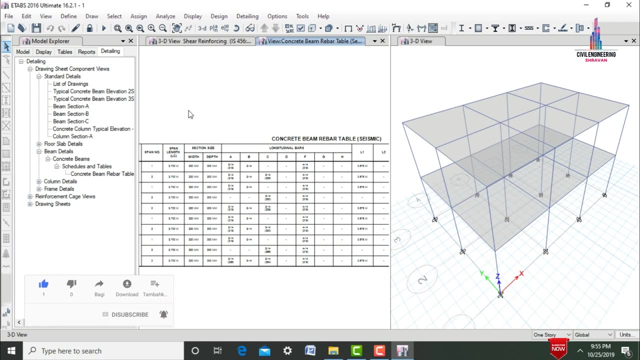 So this is the column section dimensions rebar values for this respected column section A. Select the beam detailing concrete beams. select your scheduling. Just we need to select the Concrete beam rebar table, so just double click on it. So this is the concrete beam rebar table for this respective zone, which is consisting: 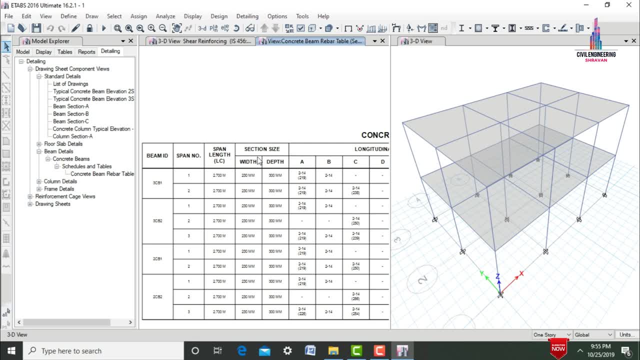 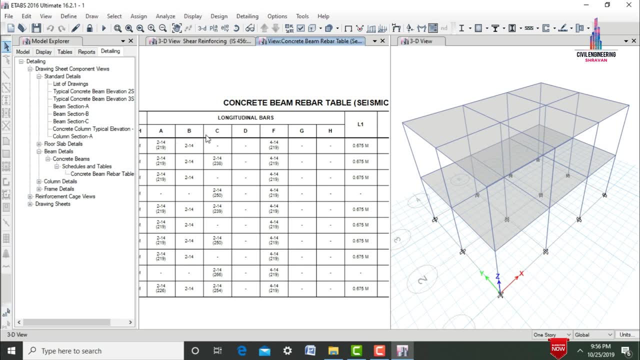 of beam ID: span number, span length, section size. So it will be consisting of the longitudinal bars, section dimensions for the respected section a, b, c, d, f, g, h, like this: So it will be consisting of two bars of 14 mm. dia 2: 1, 9 is the reinforcement value. AST requirement. 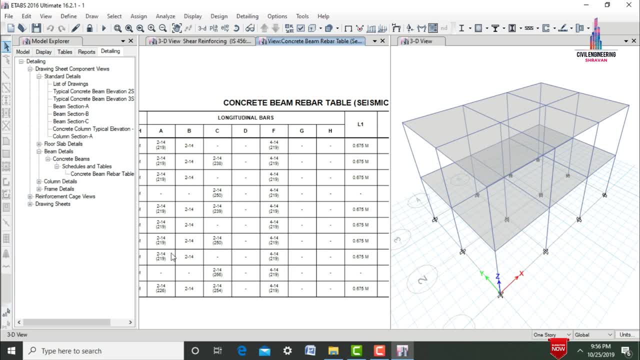 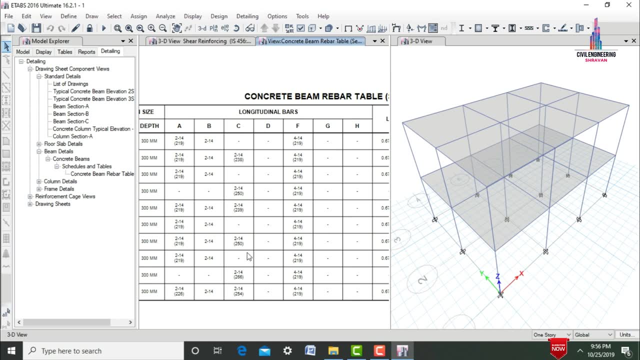 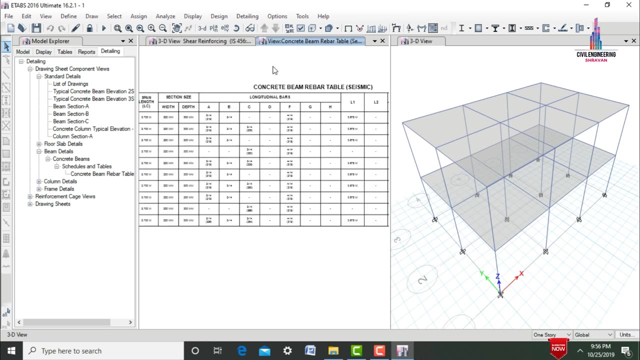 AST requirement. this respected section of a at different levels. so after that, this is the b values reinforcement detail. so it will be consisting of two bars of 14 mm. so this is the values of the c section. this is the values of the d section. this is the values of the f section. so after that we need to see the. 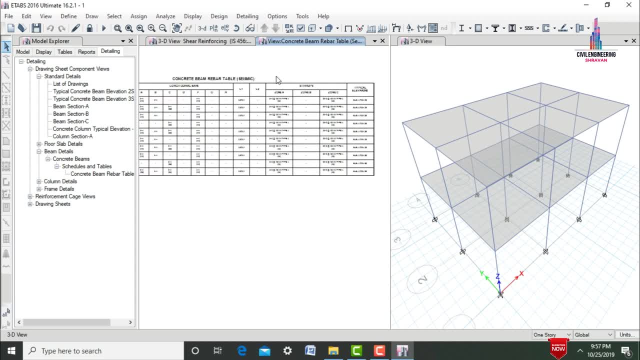 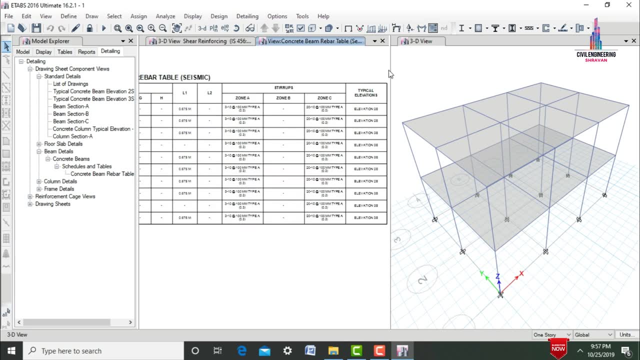 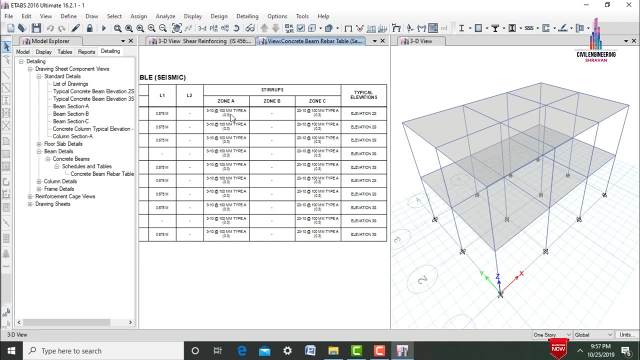 values of the zones for the beam design calculations. so this is the values of the zone calculation results for this respected stress section. so this is nothing but your stirrup section. so this is the value set zone a, which is consisting of three bars of 10 mm dia, 100 mm center to center distance. 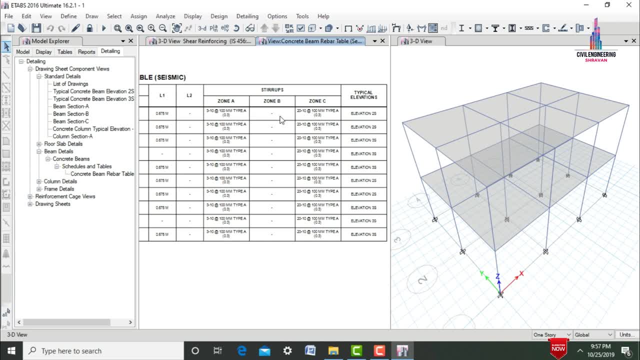 for this respected section. so this is the zone b values as well as this is the zone c values, which is consisting of 20 bars of 10 mm dia and 100 center to center distance for this typical section, for the 2a section, as well as 3a section for this respected different types of beam section. 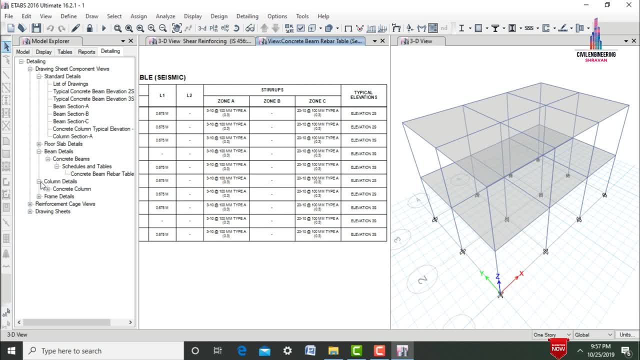 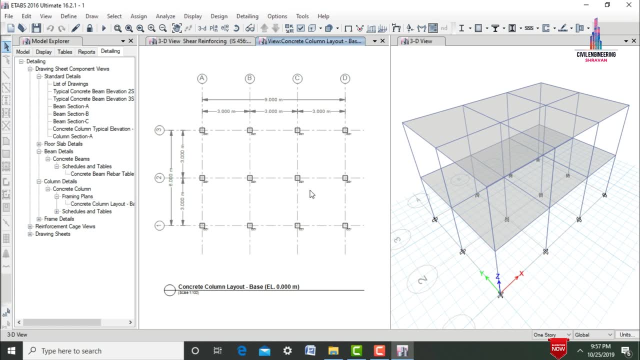 so after that we need to select the column detailsing, so select your columns. select your framing section, so just select your column layout. so this is the center to center distance layout plan for this respected column sections. so it will be consisting of 4 multiplied by 3, nothing but your 12 number. 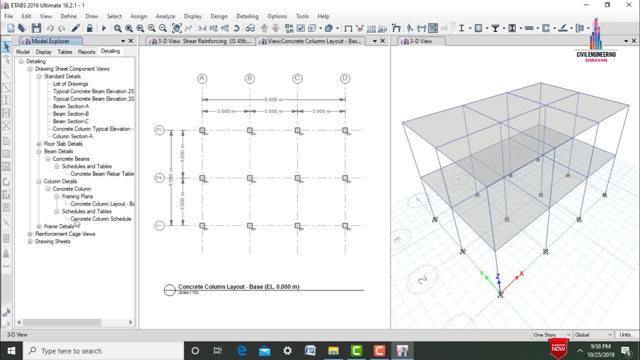 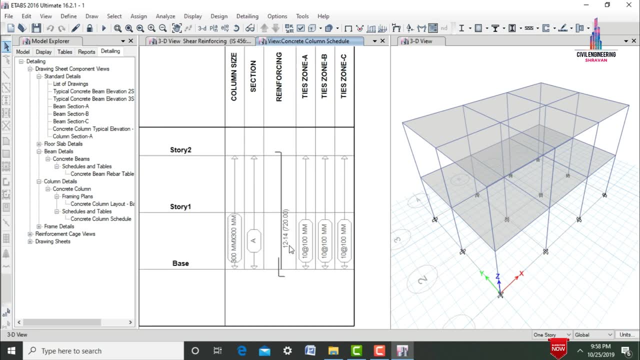 of columns. select your schedules and tables. select concrete column scheduling. so this is the concrete scheduling column for this respected section. so it will be consisting of 12 bars of 14 mm dia and 720 mm square. is the reinforcement values for this respected column section for whole building. 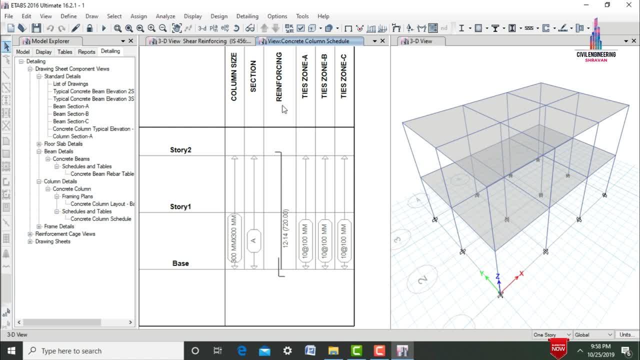 so this is the values of the column size and section and reinforcing values. ties zone for the respected values head to a, b, c. so this is the values of tie zone a to a. so it will be consisting of 10 mm dia bar and 100 center to center distance. so it zone b, also consisting of 10 mm bars, 100.